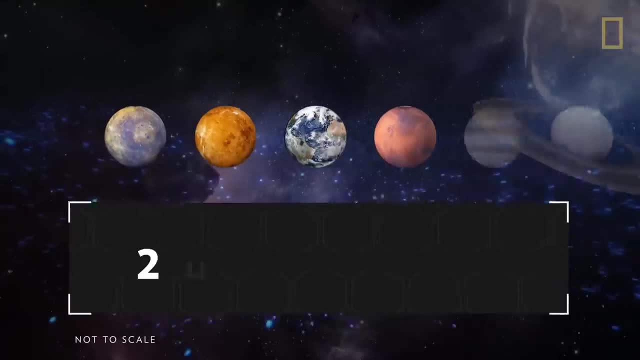 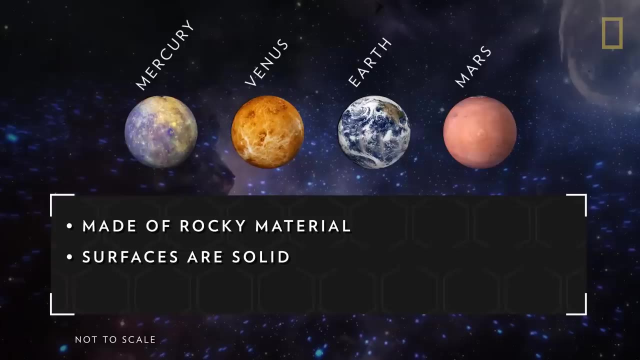 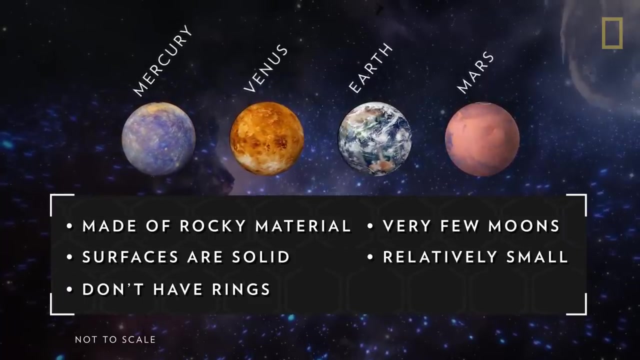 their composition, terrestrial and Jovian Terrestrial planets, including Mercury, Venus, Earth and Mars, are primarily made of rocky material. Their surfaces are solid, they don't have ring systems, they have very few or no moons and they are relatively small. The smallest and closest to the Sun is Mercury, which has 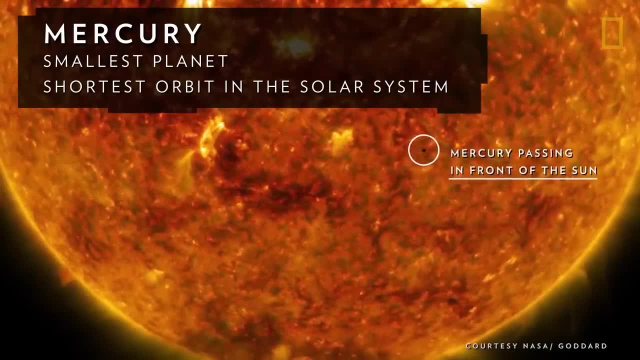 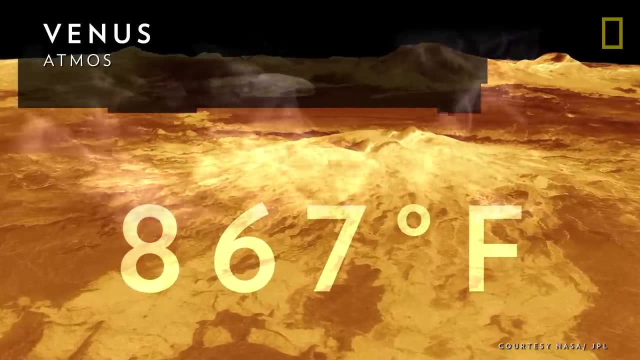 the shortest orbit in the solar system, at about three Earth months. Venus is the hottest planet, with temperatures of up to 867 degrees Fahrenheit due to an atmosphere of carbon dioxide and extensive lava flows. Next to this world of fire is a world of water. 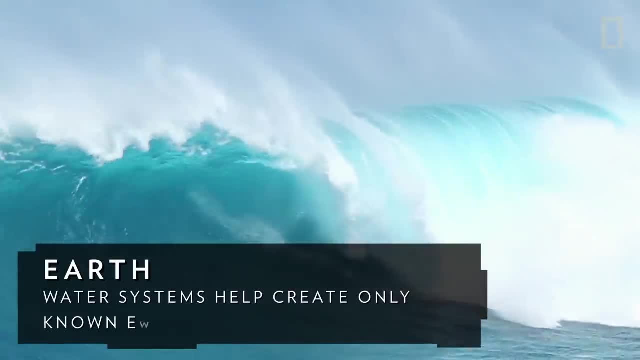 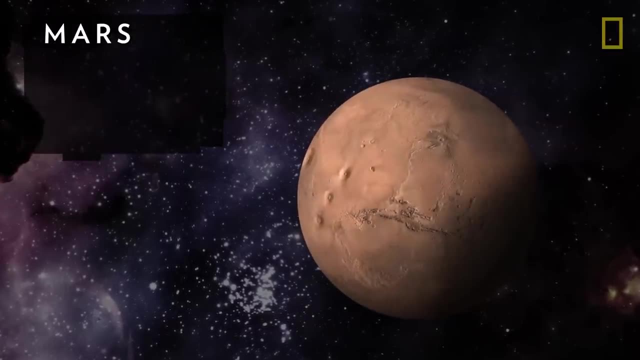 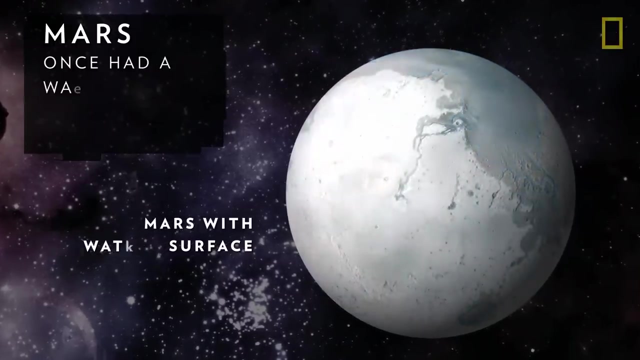 Earth. The water systems on this planet help create the only known environment in the universe capable of sustaining life. The last of the terrestrial planets, Mars, might have also supported life about 3.7 billion years ago, when the planet had a watery surface and moist atmosphere. Beyond the four terrestrial planets of 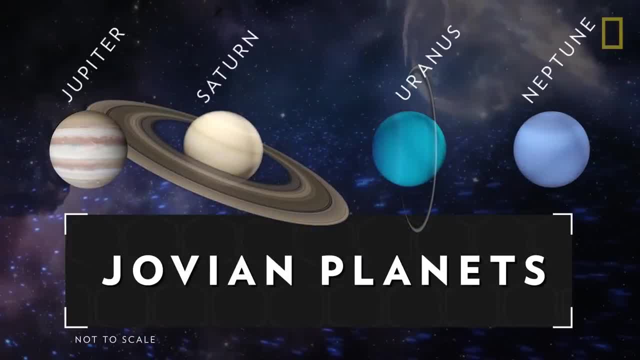 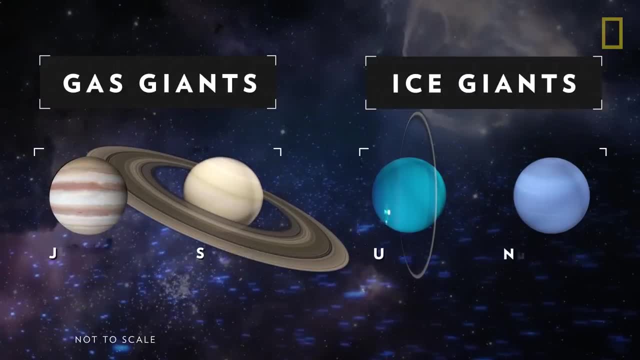 the inner solar system lie the Jovian planets of the outer solar system. The Jovian planets include gas giants, Jupiter and Saturn, and ice giants Uranus and Neptune. The gas giants are predominantly made of helium and hydrogen, and the ice giants also contain 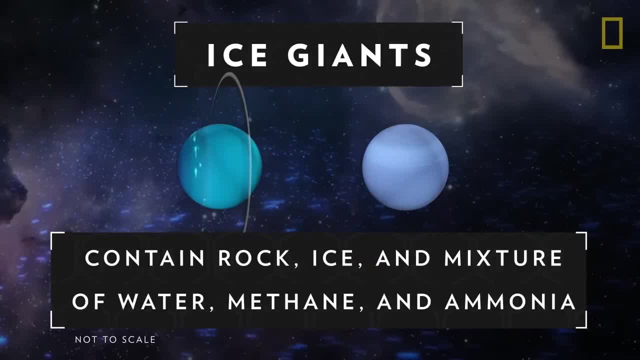 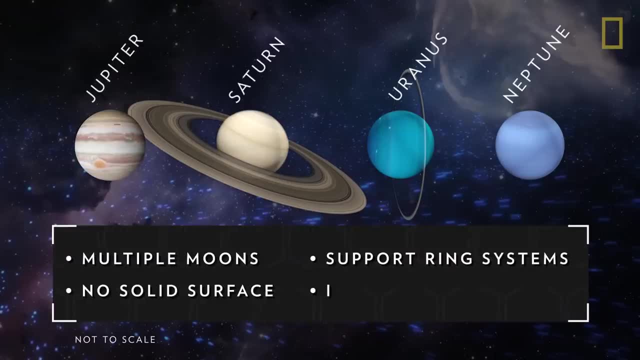 rock ice and a liquid mixture of water, methane and ammonia. All four Jovian planets have multiple moons sport ring systems, have no solid surface and are immense. The largest Jovian is also the largest planet in the solar system. 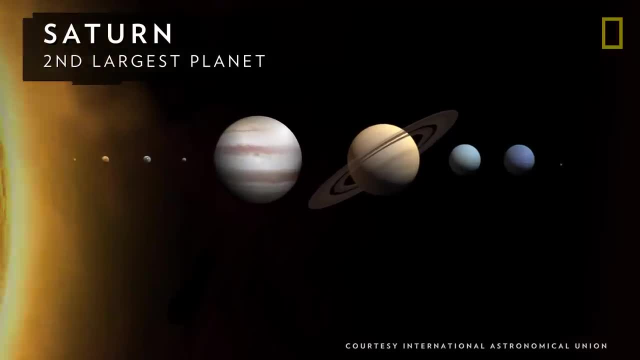 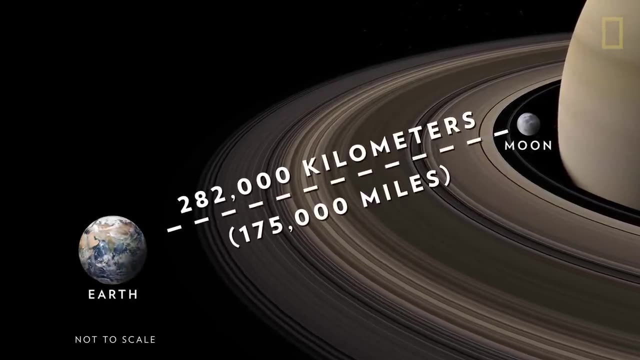 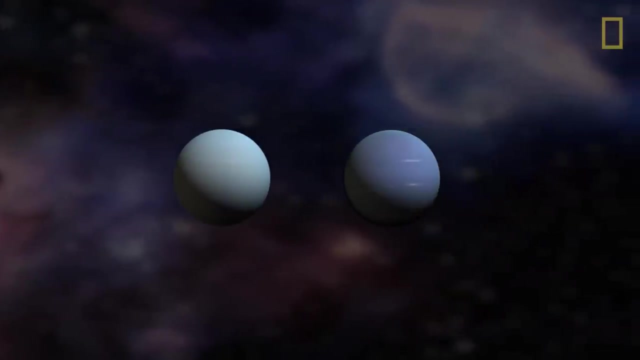 Jupiter. Next to this world of fire is Saturn, the solar system's second largest planet. Its signature rings are wide enough to fit between Earth and the moon, but are barely a kilometer thick. Past Saturn are the ice giants Uranus and Neptune, The slightly bigger of these. 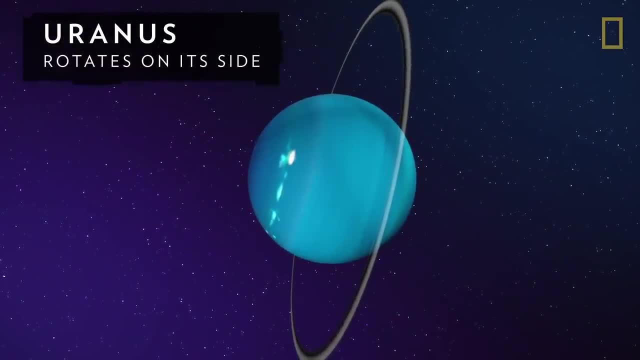 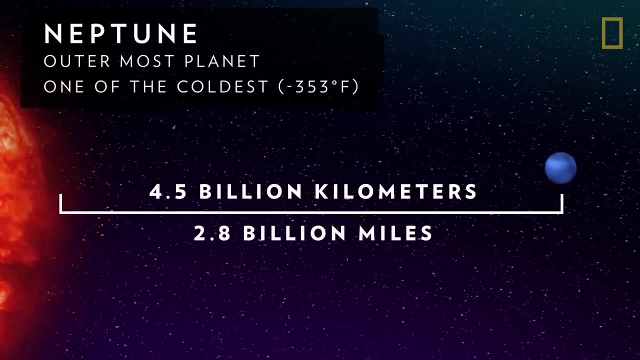 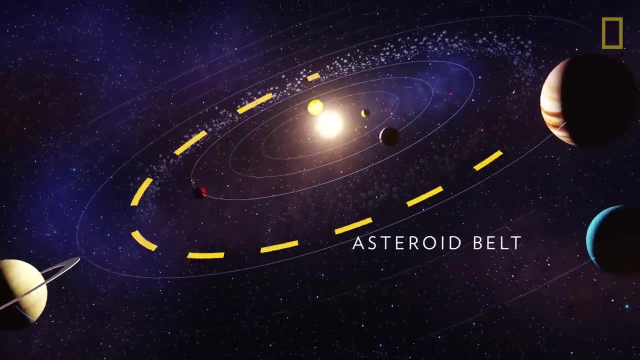 ice giants. Uranus is famous for rotating on its side. Next to Uranus is Neptune, the outermost planet in the solar system and also one of the coldest. Orbiting the terrestrial planets is the asteroid belt, a flat disk of rocky objects full of remnants from the solar 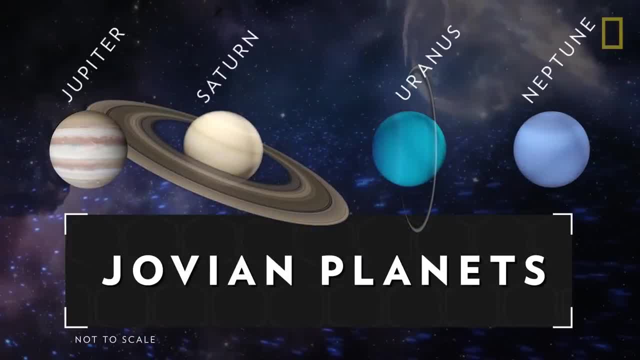 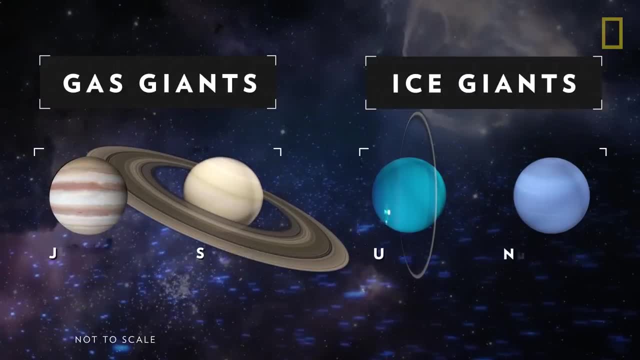 the inner solar system lie the Jovian planets of the outer solar system. The Jovian planets include gas giants, Jupiter and Saturn, and ice giants Uranus and Neptune. The gas giants are predominantly made of helium and hydrogen, and the ice giants also contain 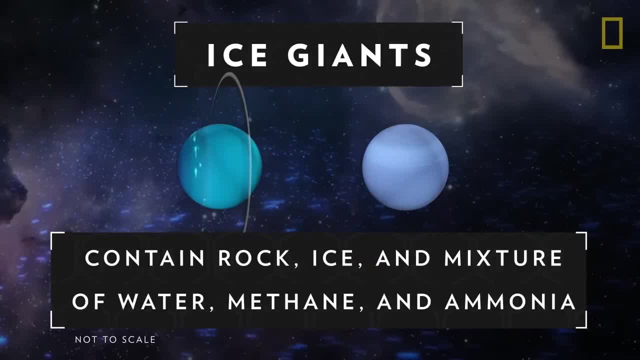 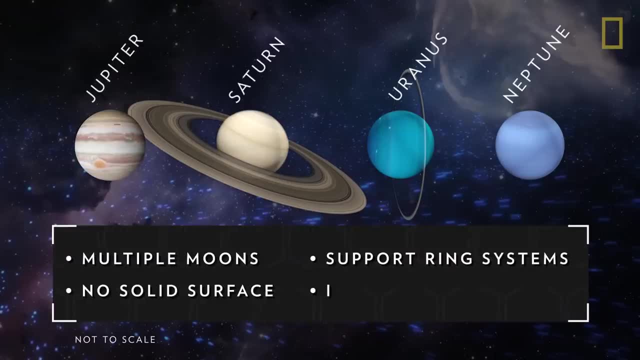 rock ice and a liquid mixture of water, methane and ammonia. All four Jovian planets have multiple moons sport ring systems, have no solid surface and are immense. The largest Jovian is also the largest planet in the solar system. 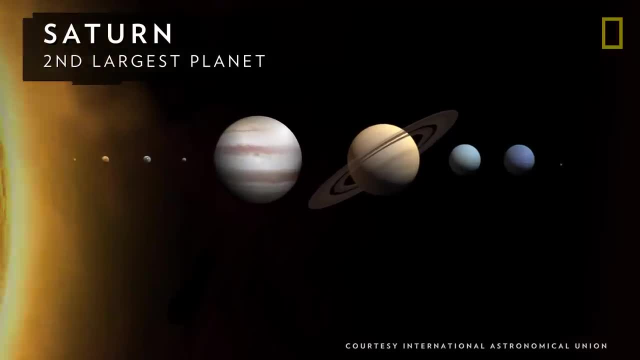 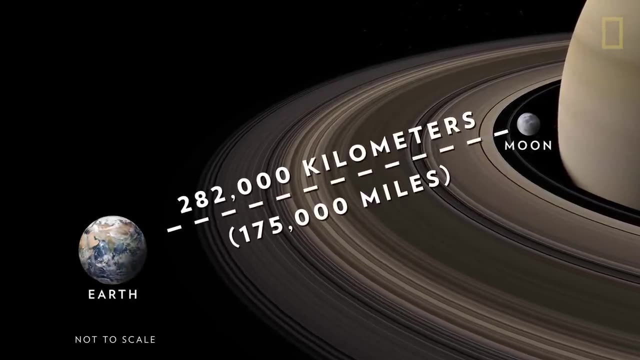 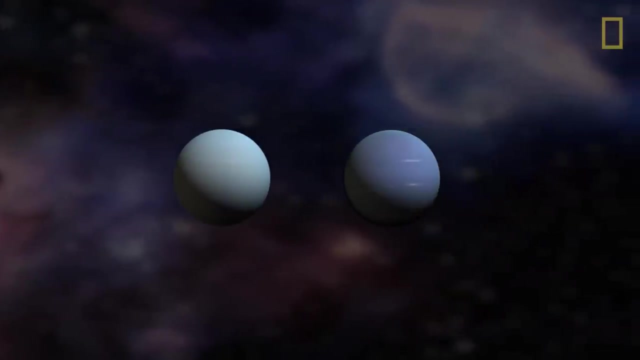 Jupiter. Next to this world of fire is Saturn, the solar system's second largest planet. Its signature rings are wide enough to fit between Earth and the moon, but are barely a kilometer thick. Past Saturn are the ice giants Uranus and Neptune, The slightly bigger of these. 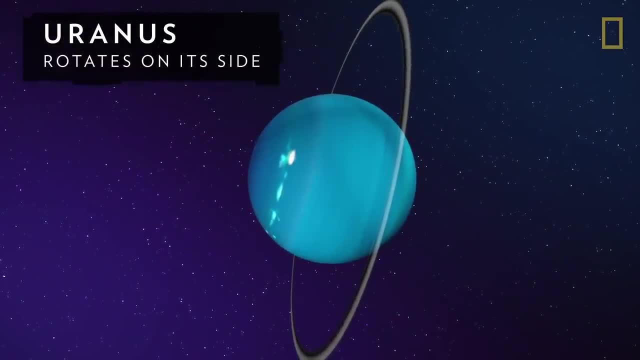 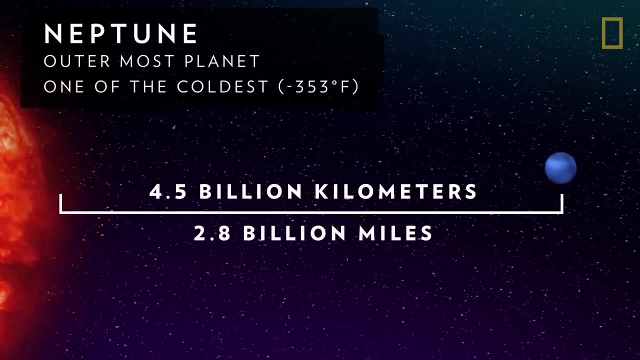 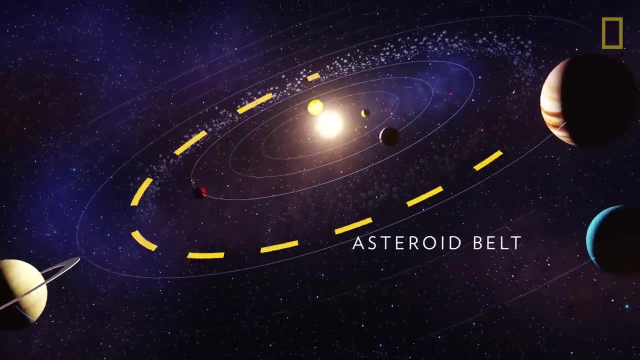 ice giants. Uranus is famous for rotating on its side. Next to Uranus is Neptune, the outermost planet in the solar system and also one of the coldest. Orbiting the terrestrial planets is the asteroid belt, a flat disk of rocky objects full of remnants from the solar 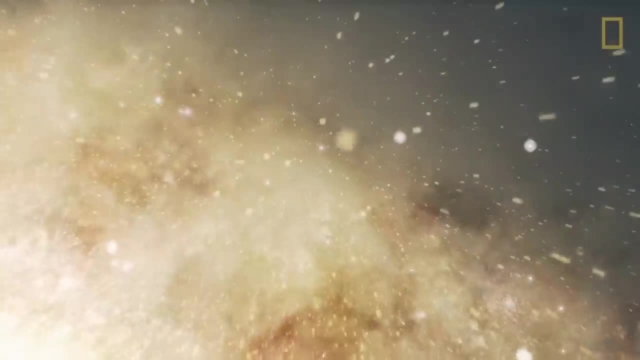 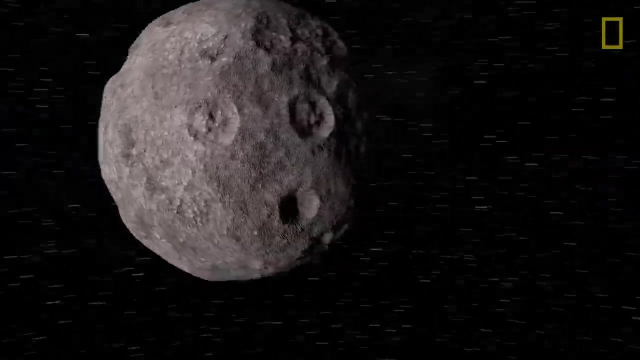 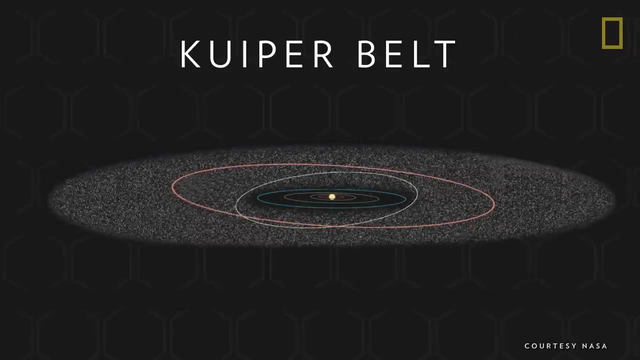 system's formation, from microscopic dust particles to the largest known object, the dwarf planet Ceres. Another disk of space debris lies much further out and orbits the Jovian planets: the icy Kuiper belt. Apart from asteroids, the Kuiper belt is also home to dwarf planets such as Pluto and is the birthplace of many comets. 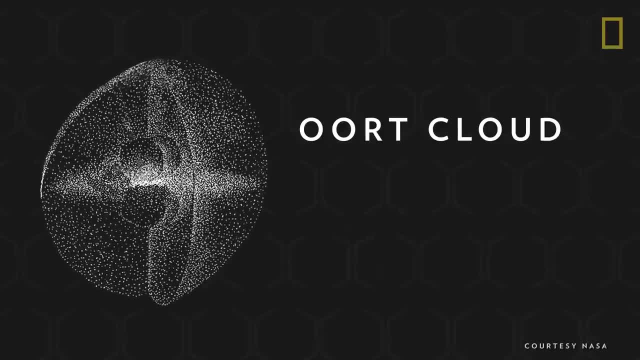 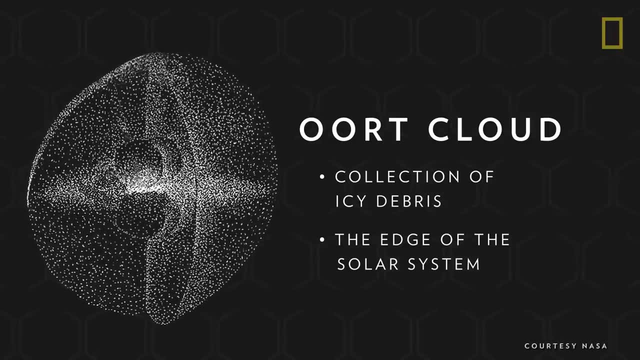 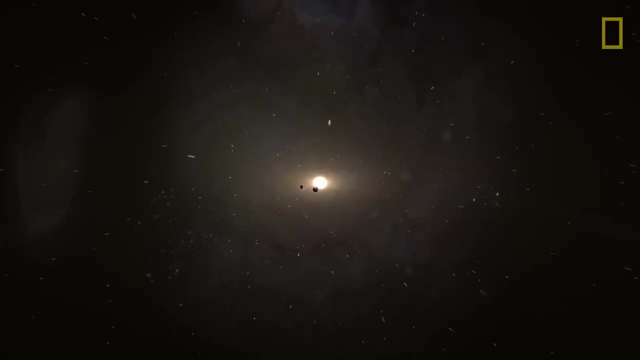 Beyond the Kuiper belt is the Oort cloud, a vast spherical collection of icy debris. It is considered the edge of the solar system, since that is where the gravitational and physical influences of the sun end. Our solar system's particular configuration of planets and other celestial objects, all revolving around a life-giving star, make it a special place to call home. 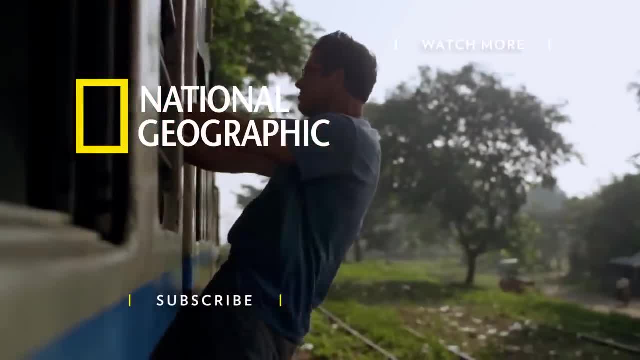 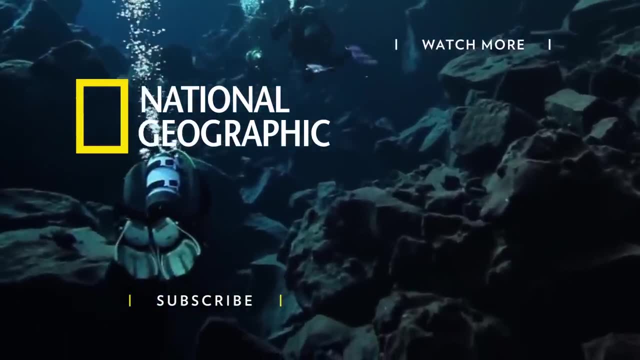 The Oort cloud is one of the most abundant planets in the world. It is a natural asteroid, and it has been treasured for over 300 years. In the dissevered Oort cloud, or the Earth's first ozone layer, you will find星et cycles of each of its own. TheAKR is the world's most treasured object. TheKUAD is the world's most treasured object.